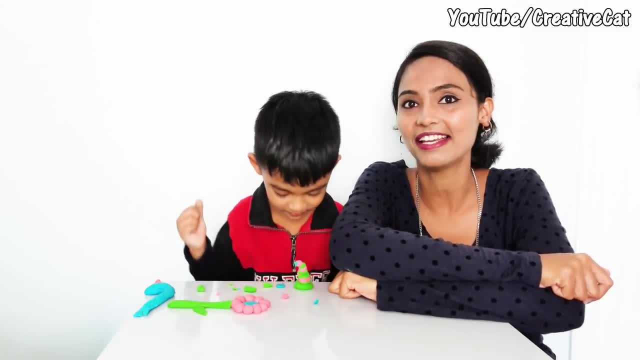 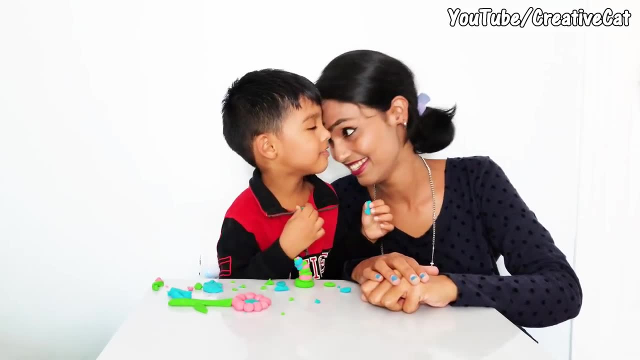 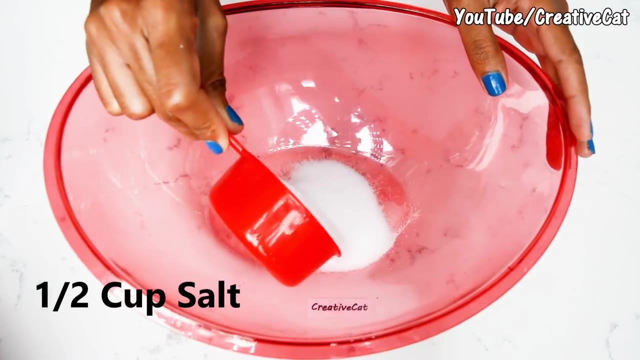 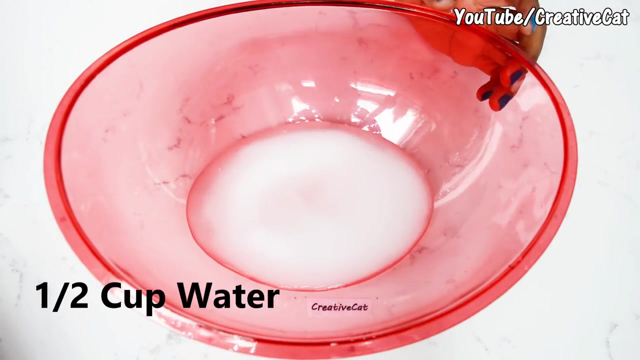 Let me know in comments what you think about it and do subscribe to this channel for more videos like this. Let's see the recipe. I am taking 1⁄2 cup of salt, 1⁄2 cup of water. Try to dissolve salt in water. 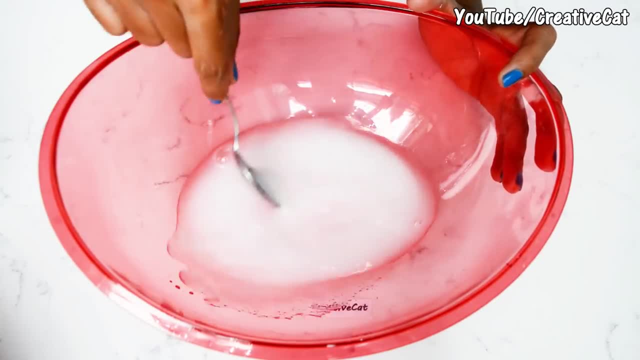 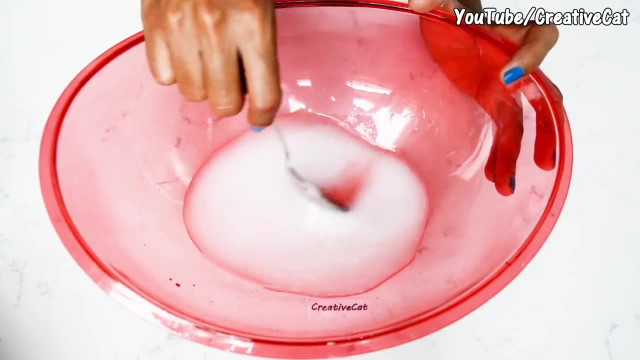 It won't get dissolved easily as the salt amount is really high, But try to dissolve as much as you can. as it really affects the Play-Doh texture and makes it grainy, I am adding 1 cup of all-purpose flour or maida. 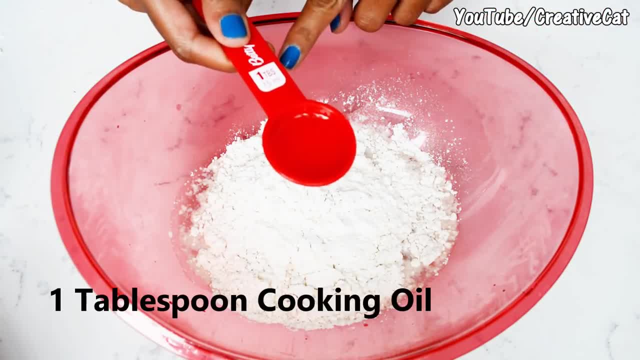 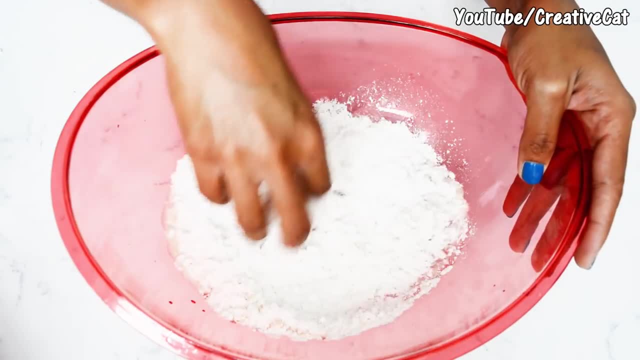 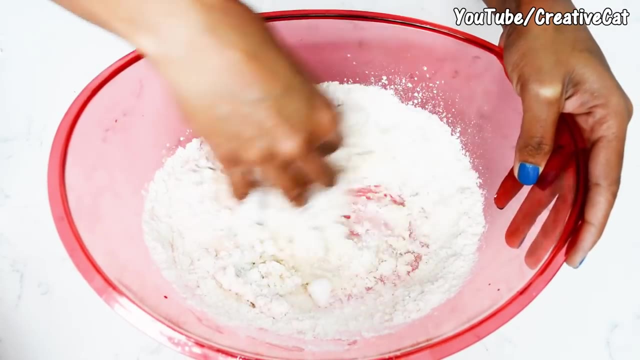 Mix it well, And this is 1 tablespoon of cooking oil. Mix it well. The high salt content works as preservative. It's all non-toxic ingredients, though Still advise your kids not to eat it, as excess salt can be harmful to their health. 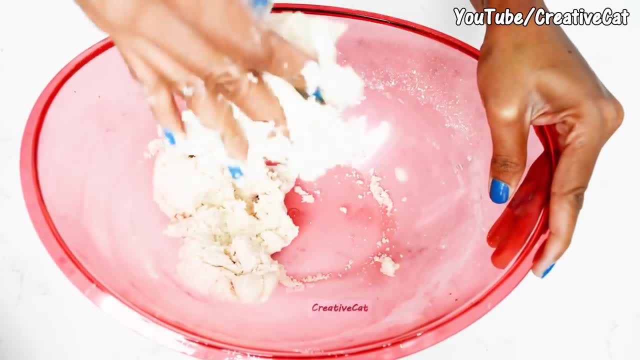 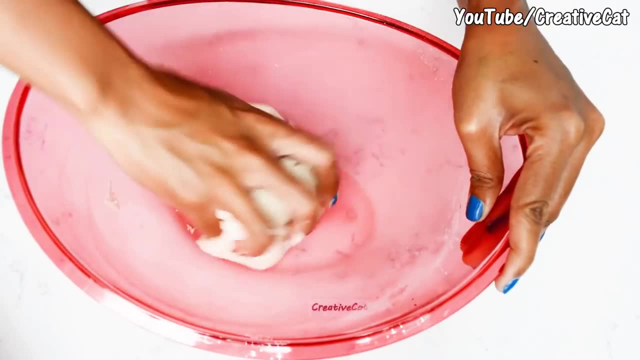 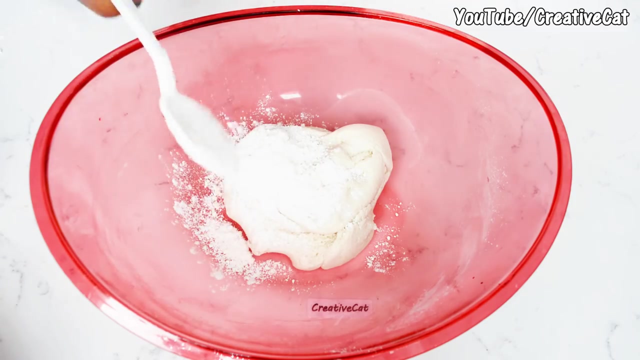 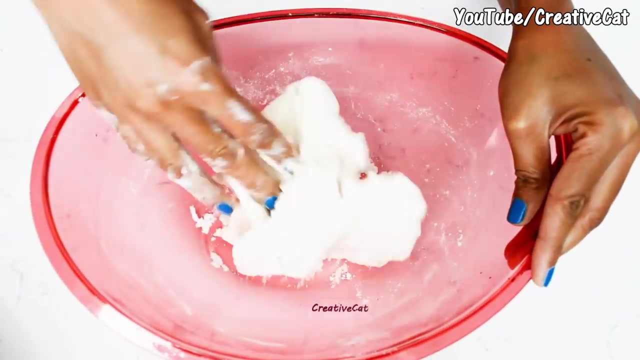 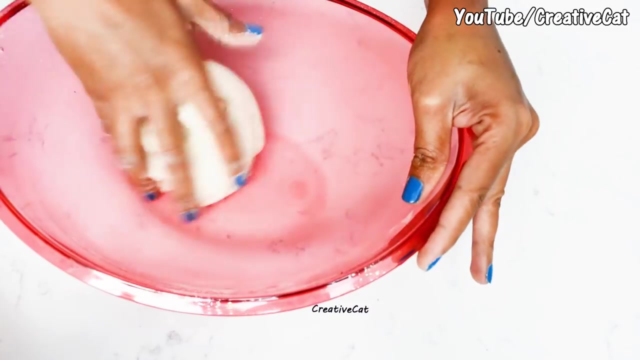 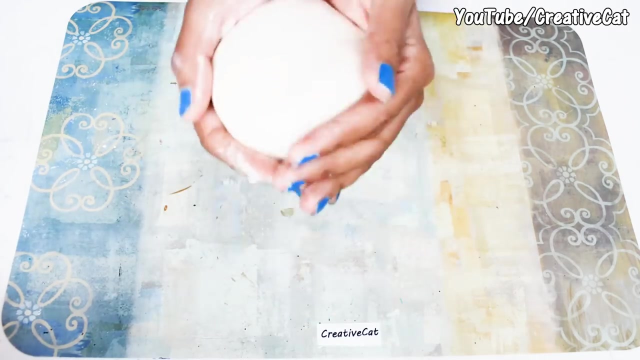 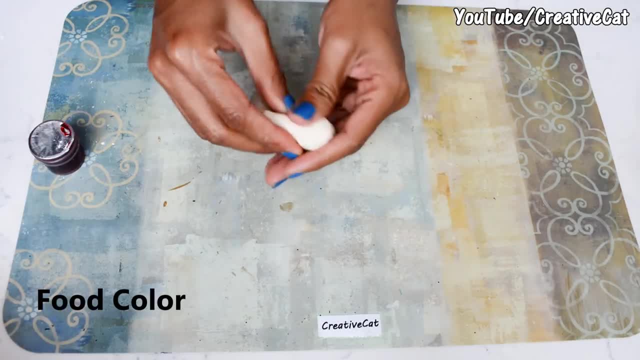 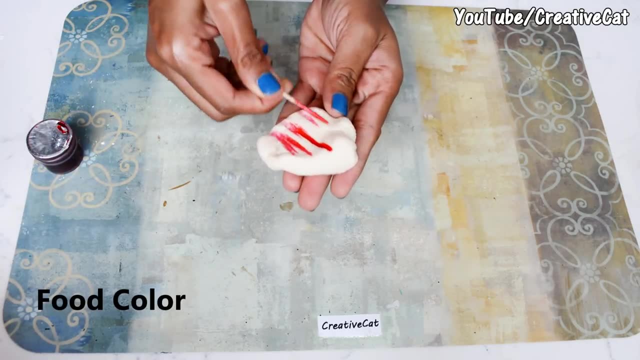 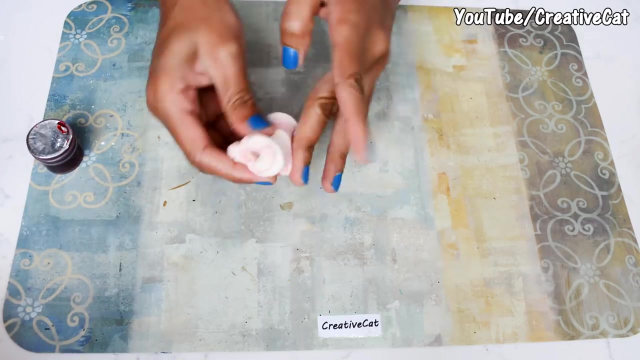 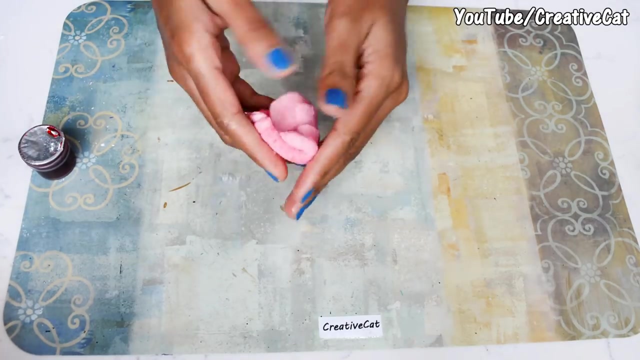 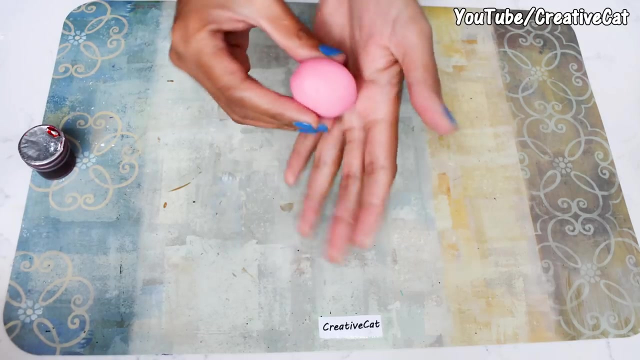 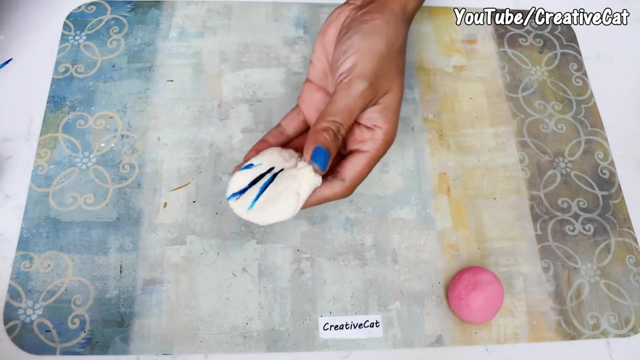 This is pink food color. You can either use gel color or dry colors. Liquid colors will make the clay soft. I will advise you to strictly use food colors. only Mix well. You can apply little oil on your hands. Coloring this blue.